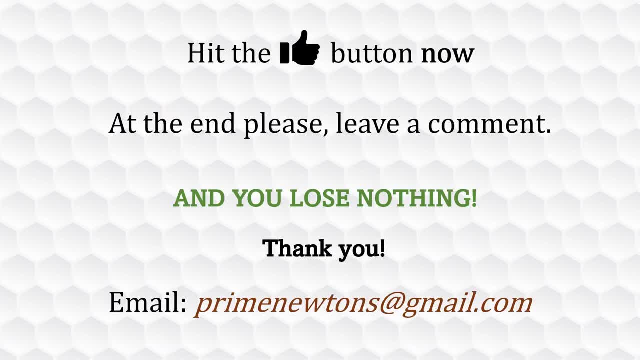 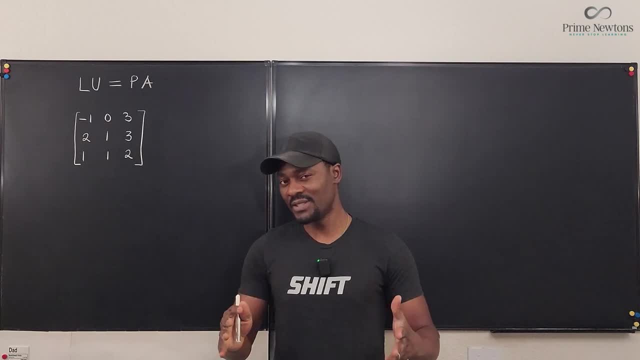 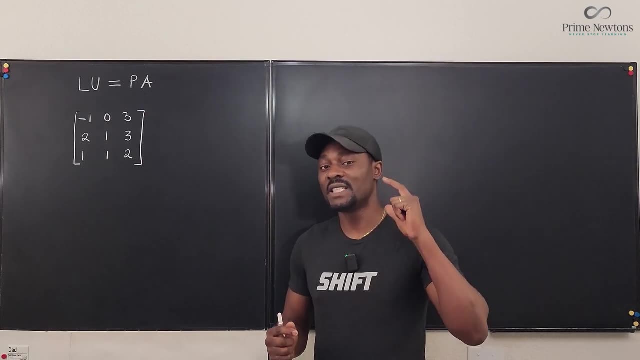 Welcome to another video. I will continue the series on linear algebra and matrices, and today I want to talk about matrix decomposition. I want you to look at a matrix for this video as the number 12.. You could write 12 as 12 times 1, right. And you could also write it as 6 times 2.. 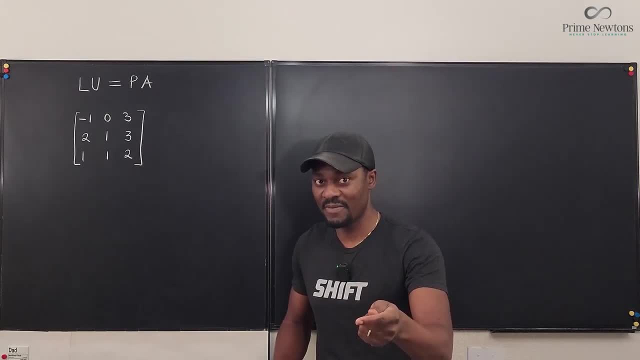 You could also write it as 4 times 3.. That's how I want you to view this equation. Look at this matrix. Let's say this is A. If this is A, then you would expect this P to not make any changes to A. 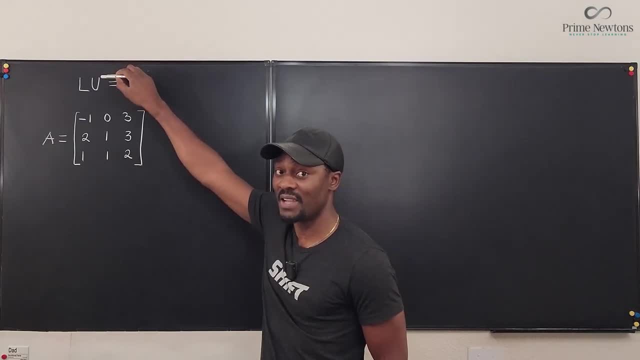 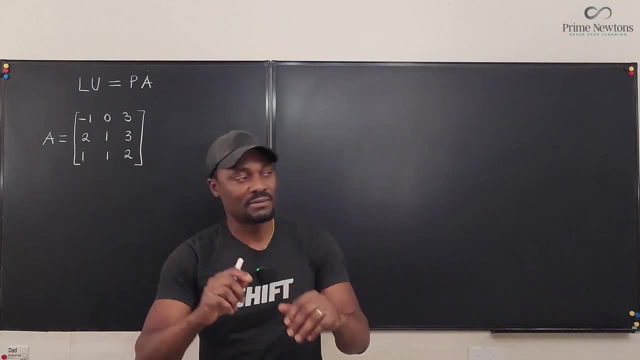 if you're going to retain the same value on the other side, especially if you want the product of these two to retain the value of A. So this is what I mean. Imagine that 12 times 1,- let's say 1 times 12, is the same thing as 4 times 3.. In your head you could look at this as P times A is L. 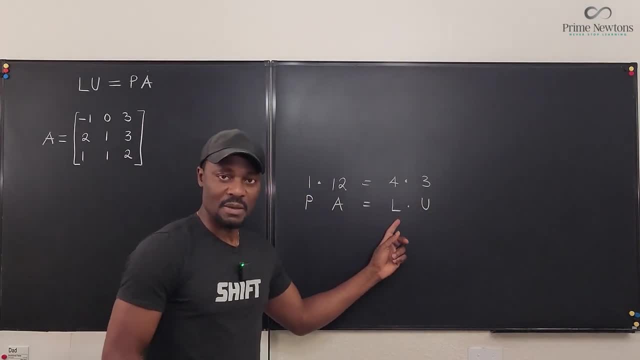 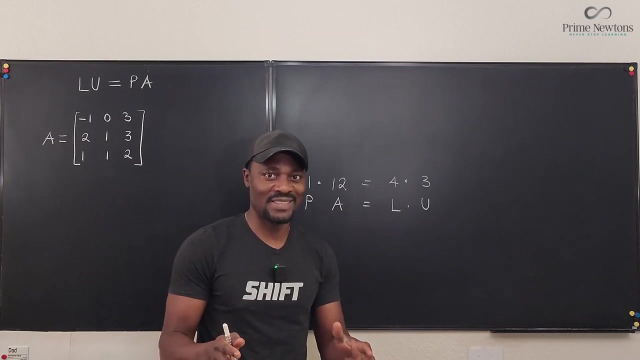 times U, Where L is a matrix, U is a matrix, A is a matrix and P is a matrix, You can actually write a matrix as a product of two matrices. It's just a special case. And that special case is where what we call 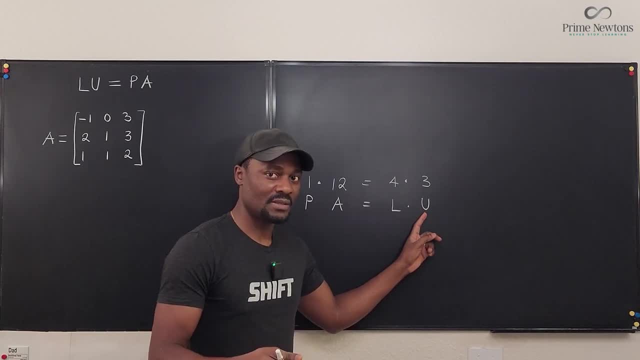 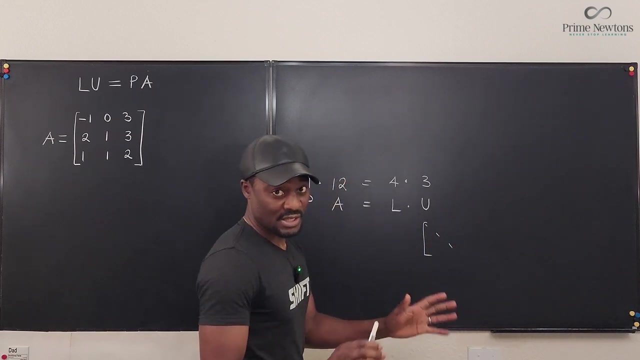 U is an upper triangular matrix which we can obtain by doing elementary row operations on the original matrix and obtaining an upper triangular matrix which looks like this. Typically, an upper triangular matrix is going to look like this: You're going to have numbers or not, not zeros, but you. 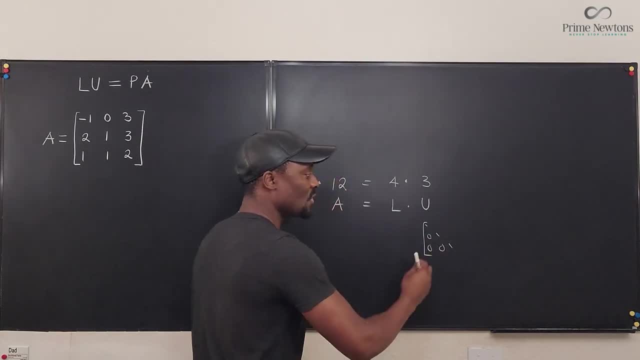 definitely will have zeros down here, So that where you have all the certain zeros will be under diagonal. You certainly will have zeros here. And this is what you do when you do Gaussian elimination, Remember, Because all you're doing is generating as many zeros on the bottom so that you could get your answers on the 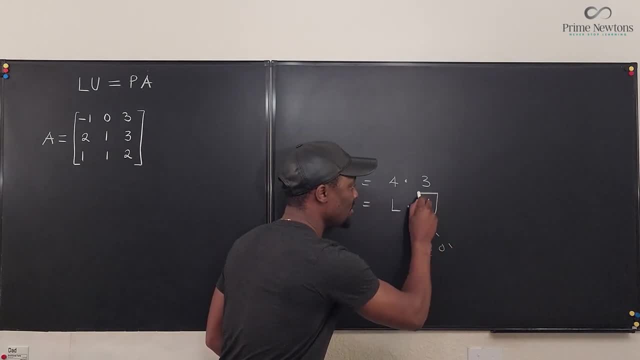 right. So this is a very important matrix. U because this U, we named it U because it is called the upper triangular matrix, form of A. So you would ask me then, what is L? Well, just as U is upper triangular, L is: 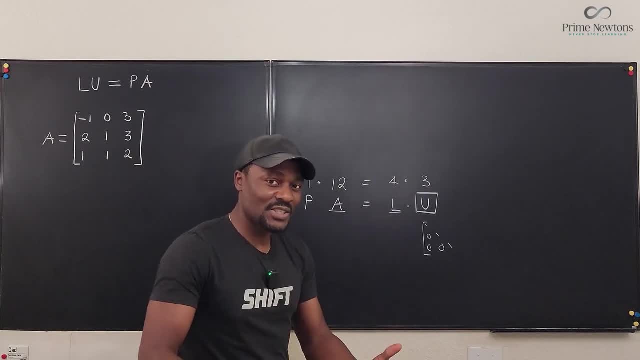 the lower triangular matrix simultaneously generated from the elementary row operations we're going to be performing. and this is what it says: if you multiply the lower triangular matrix that we obtain by the upper triangular matrix that we really need, because this is the most important thing here- then you're gonna get your original matrix back, and if it is not, the 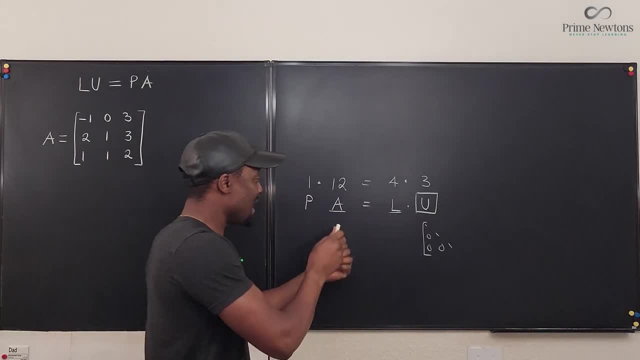 original matrix that we had. it must have been modified or permutated, and when we say permutation, it means you may have switched some rows so it doesn't look like the original matrix, and this guy will be bearing that flag telling you that. hey, remember, when you perform this elementary row operation at this. 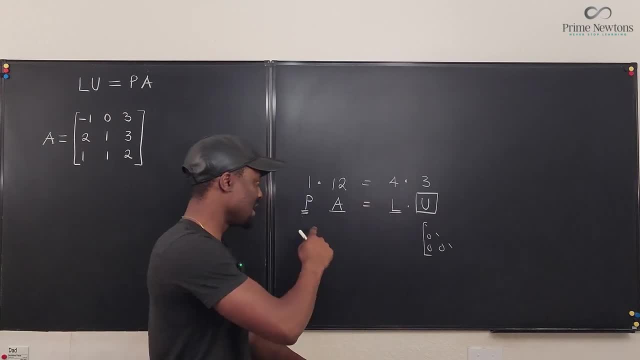 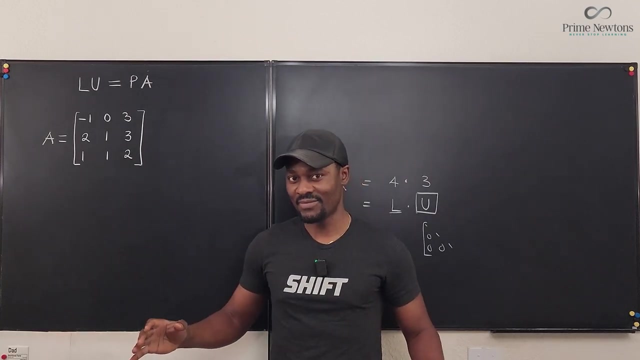 point. you switched two rows and this guy gives the evidence. otherwise this is what you're gonna get. so this is called the permutation matrix because it gives evidence that you have switched rows while performing the whole operations to obtain your upper triangular form. otherwise you'll get that. now, when I show you this example, you will see it clearly. I hope I give. 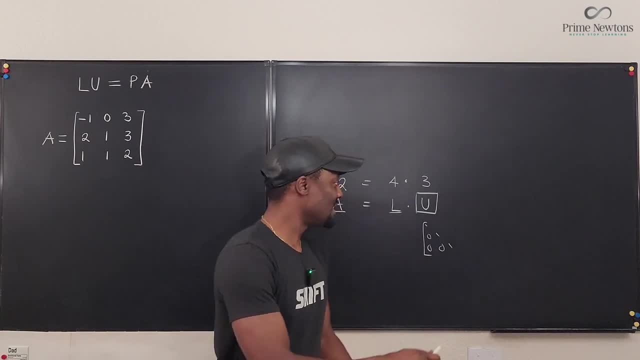 you. I gave you a very good idea of what we're gonna do. this is the most important matrix because from this matrix, which we say is gonna be well, every upper triangular form that you're going to perform is going to be the most important matrix, because from this matrix, which we say is gonna be well, every upper triangular form that 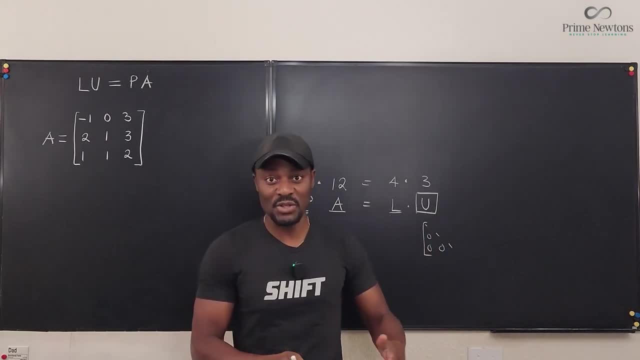 you're gonna get in this case is gonna be in the row echelon form, and the row echelon form straightaway helps you get what the rank of the matrix is, what the nullity of the matrix is. it tells you it's easy to compute the determinant of. 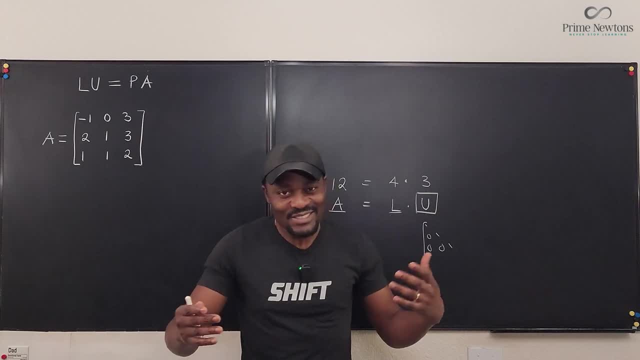 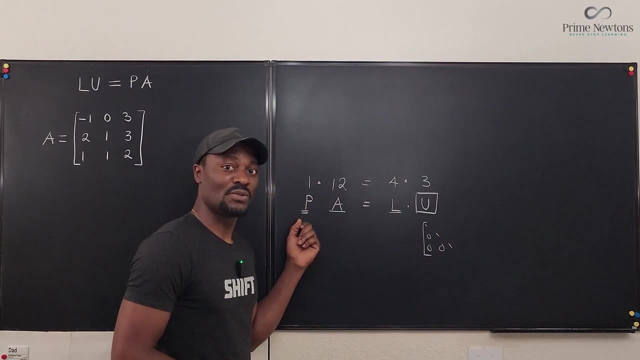 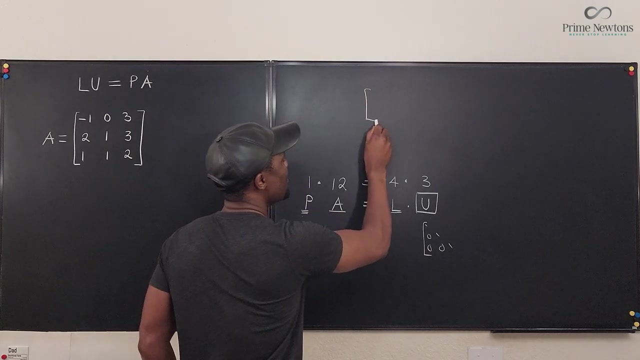 the matrix to some degree, okay, but there's so many things you can find about this and this guy has some unique properties also, and I'm going to explain it to you now. one more thing: look at this matrix. let's say I have a matrix one, two, three, four. 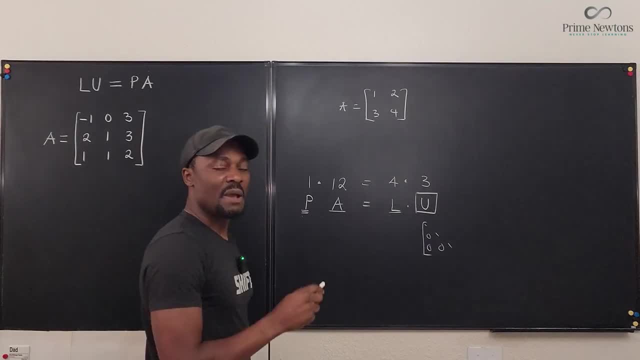 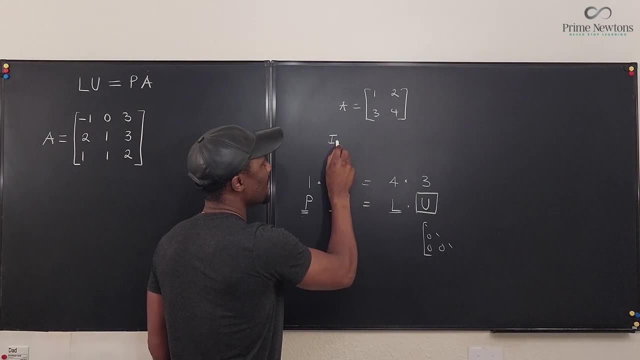 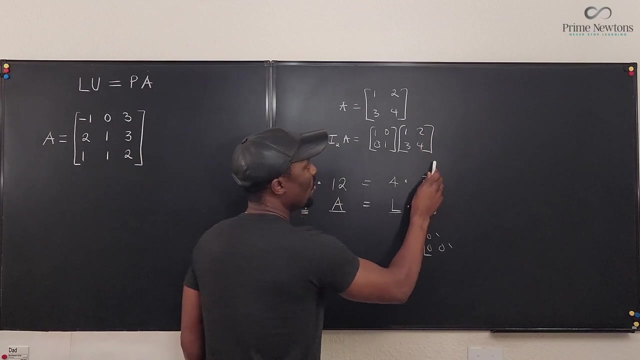 this is a. if I multiply this matrix by the identity matrix for two by two matrices, for example, if I say I for two by two matrices multiplied by a, well, my, it's just one, zero, zero. one multiplied by this matrix: one, two, three, four. well, my answer is still this: one, two, three, four. if you do this multiplication, 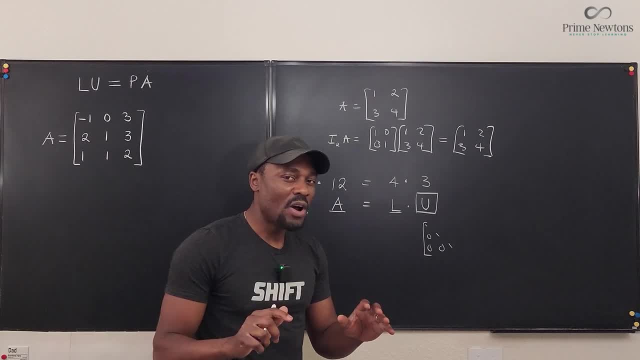 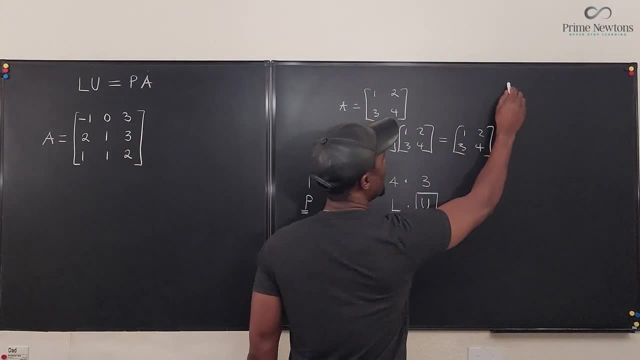 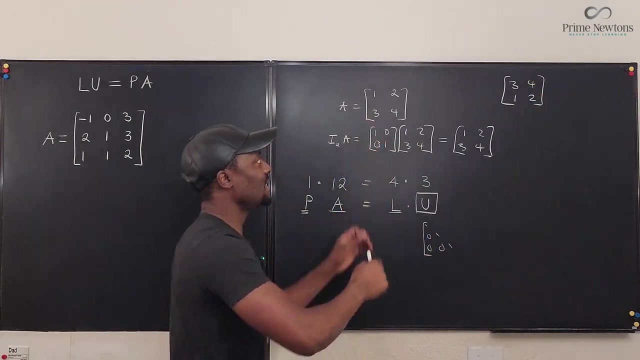 you get the same answer. but what if I want to switch the rows of this matrix? let's say I want to write: I want this to become three, four, one, two. if I don't want to act directly on a, I can as well act directly on this guy. 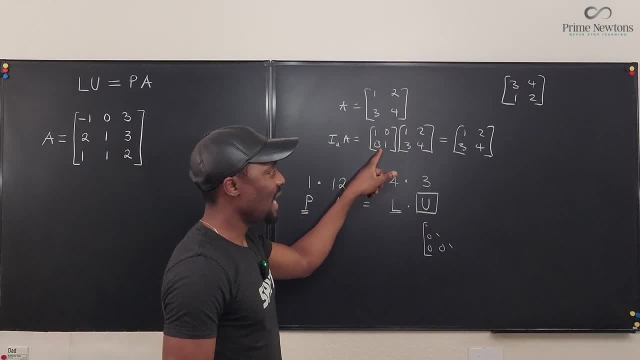 I could switch the rows in this one, okay, such that instead of multiplying this by this, I switch these rows so that this becomes zero one. this is now zero one, one, zero. if I multiply, I'm not gonna get this. this is the guy I'm gonna get, so. 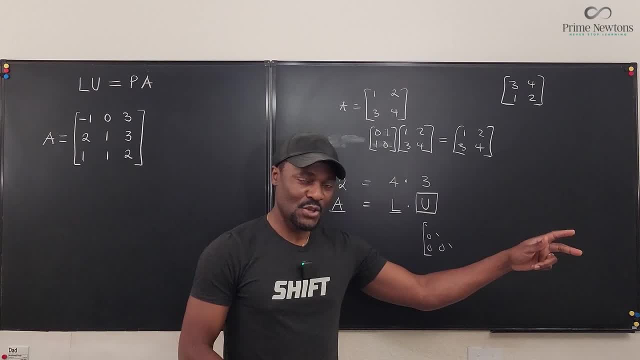 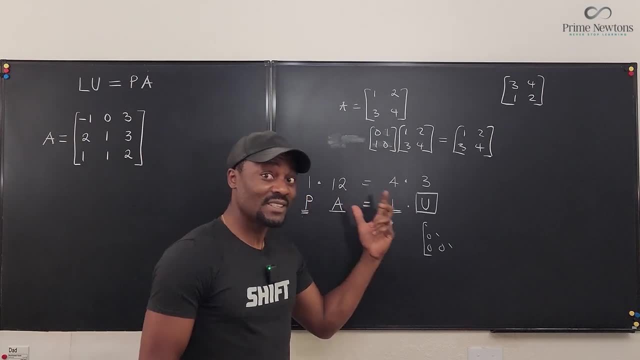 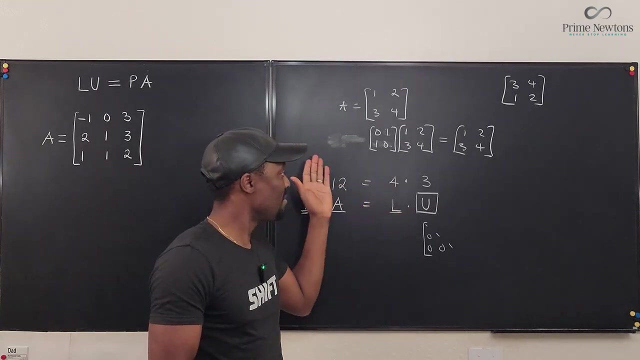 instead of actually switching the rows in a matrix, you can switch the row in this piece. this P actually is the identity matrix that we start with and if you don't touch it, it, like I said, if you don't touch it, you get back your original 12, if you touch it, it becomes maybe. 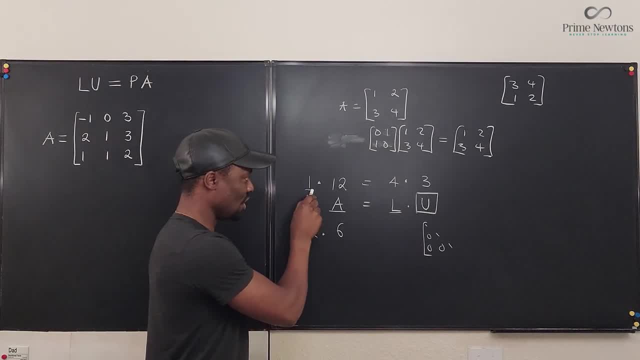 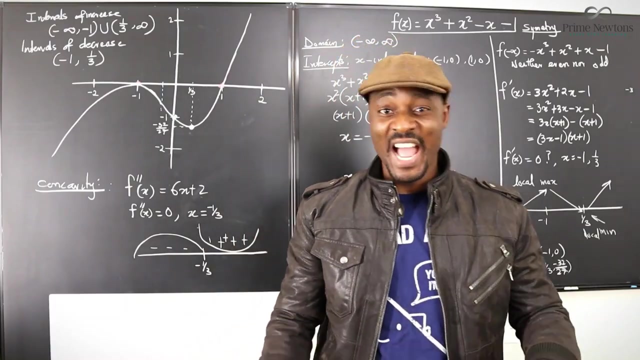 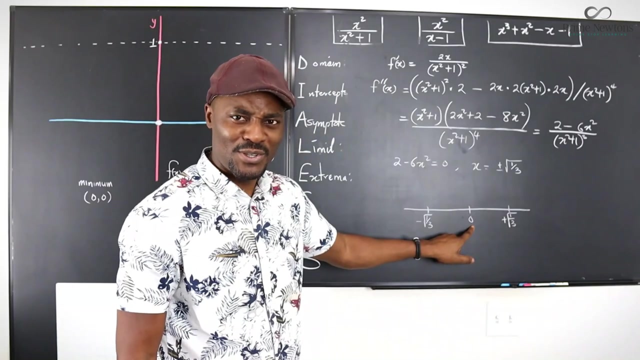 two times six. that's the modification, because you've changed the one and it has become two. then this 12 will have to change to become six, and that's the whole idea. okay, now let's get into the video. so I'm going to take the first case in which I did not switch any rows. 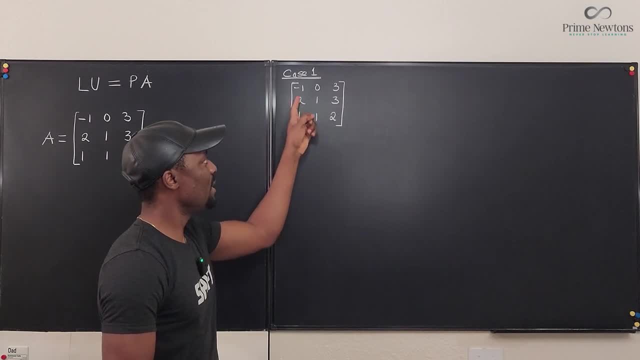 I'm just going to go straight to creating zeros below the main diagonal. that's the mission, because when you have zeros here, then you call it an upper triangular matrix, and that's how you create a matrix, and that's how you create a matrix, and that's how you create a matrix. 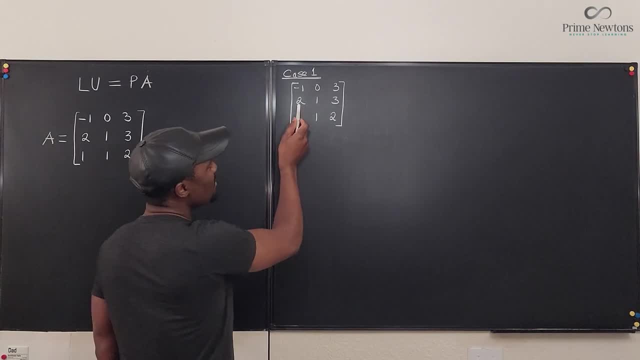 okay, so watch what's going to happen. I need to make a zero here. I need to make a zero here, so I just do the usual elementary row operations. I'm going to say that r2, the new r2, will be equal to. I need two of this to be added to this. so I need two of row one to be added to row two. 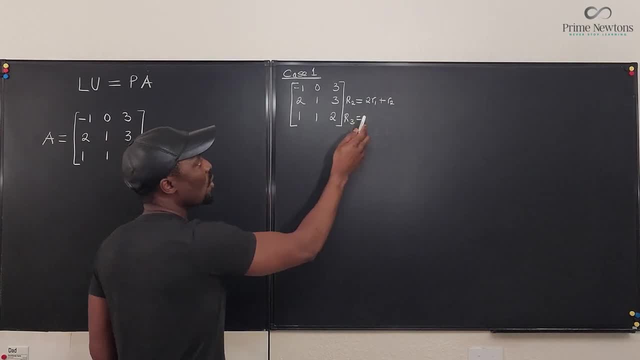 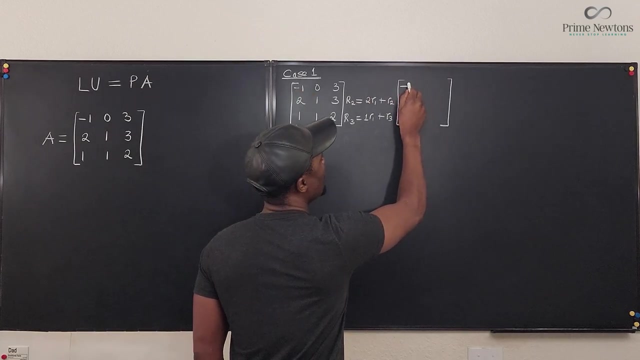 for row three. I will need one of row one, just one. make sure you write the one so you know what number you're picking. need one of this to be added to this? what do I get? I'm going to write the first row, I'm not changing it. minus one, zero, three. I'm going to write zero here I need. 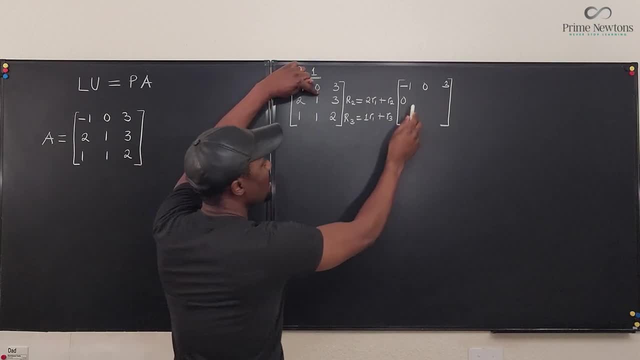 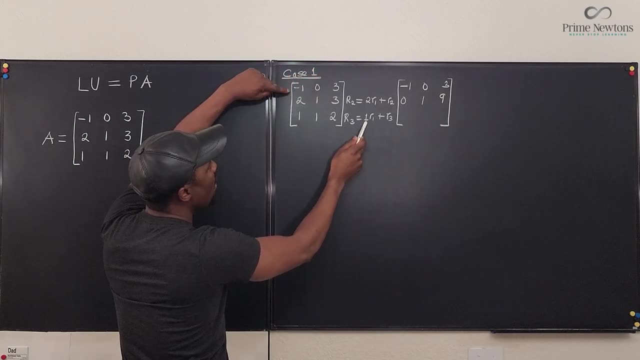 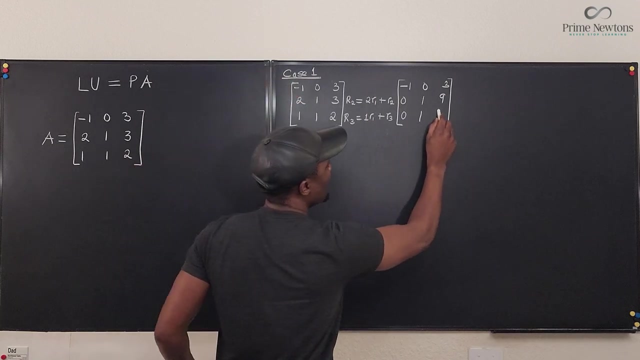 two of row one added to row two, so this is going to be one. two of this added to this is going to be nine. here I need one of row one added to this. I get a zero. one of this added to this is one, and one of this added to this is five. okay, we're almost there. we need one zero here. so 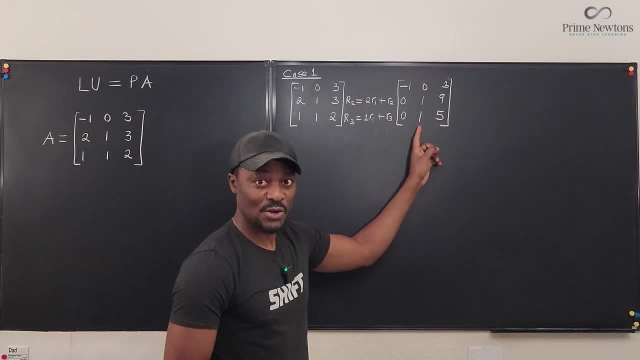 now, because I have moved to the second column, where the zero is, the pivot is the next one, so that's what you call the row echelon form. now, for row echelon form, you don't have to have a one here. it doesn't matter what number is here, as long as there's a number there, okay, there's a pivot number. 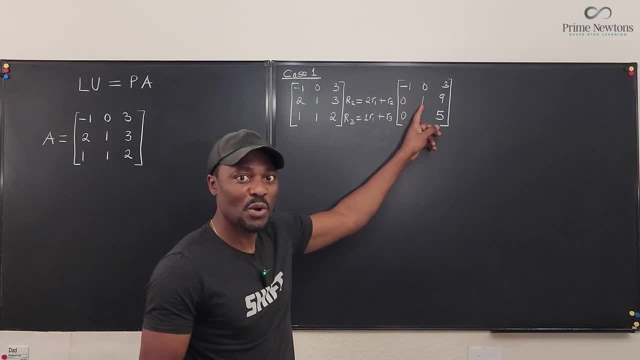 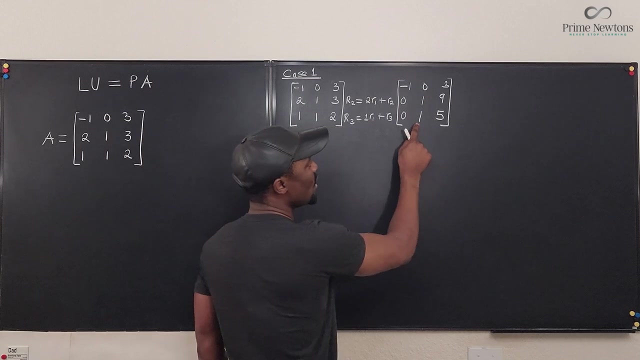 that's not zero. so here we go here. this is the second row, second column. there has to be a number there. if there's no number, we got to fix it okay, and that's where the switching may happen. but for now let's just go on. now here. I need to make a zero here. so it means what do I do? this is the. 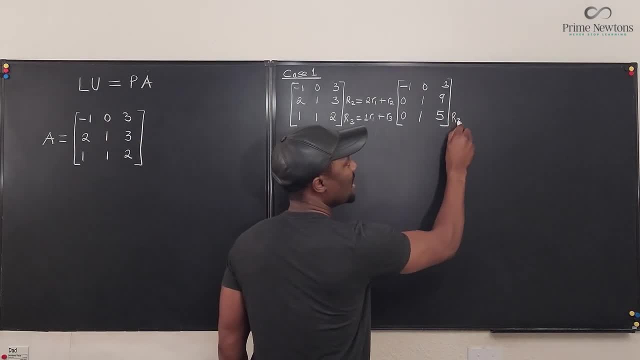 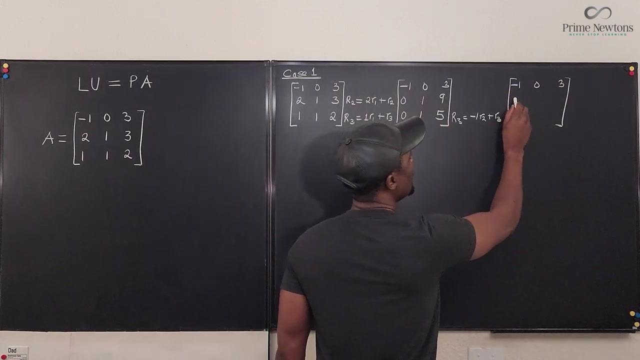 only part that I need to modify. so I'm gonna say row three is equal to. I need one of this, one of. oh, I need minus of it because I'm gonna be adding it. so I need minus one of row two added to row three. the top is gonna be minus one, zero three. here we're gonna have zero one nine and here I. 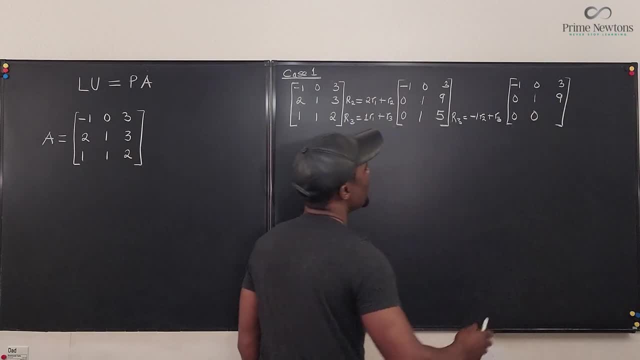 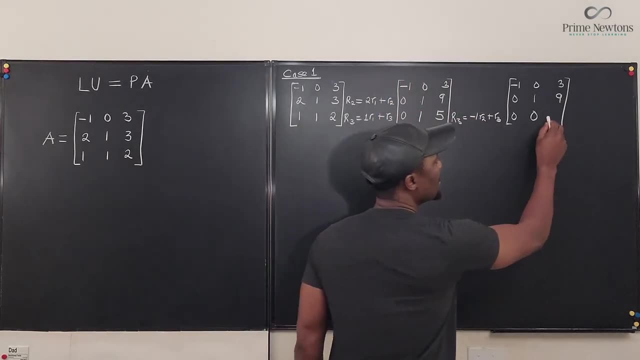 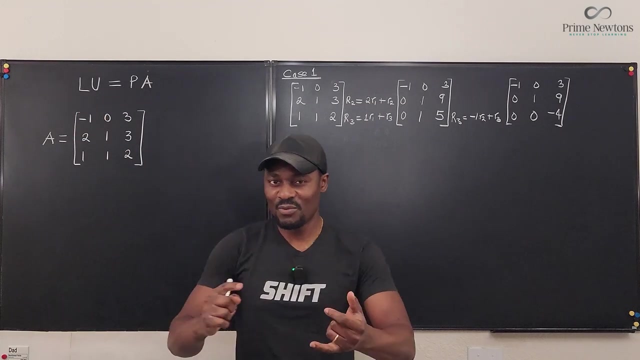 need. this is going to be zero, zero, and remember it is minus this plus this. so minus nine plus five is going to be minus four, and this is the U from this equation. then what is P, what is A and what is L? I'm about to show you all four of them in an equation. so this is your equation. 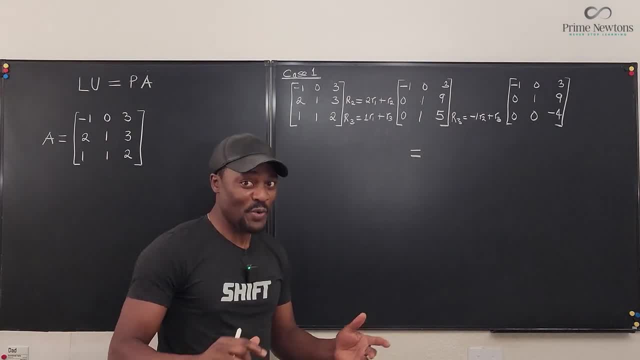 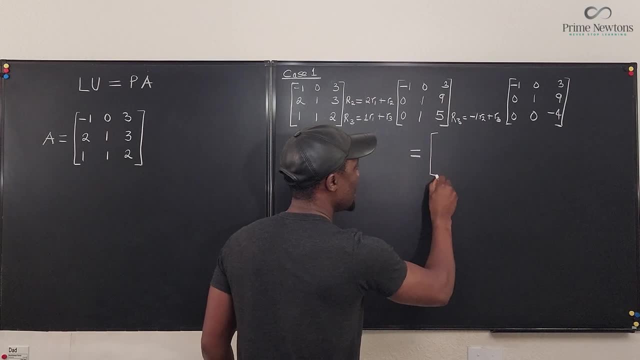 something, because we didn't switch any rows. all we did was just do addition, adding a multiple of one row to another. what you're going to have here is basically your identity matrix multiplied by the original Matrix that we're working on. so, on the left hand side, 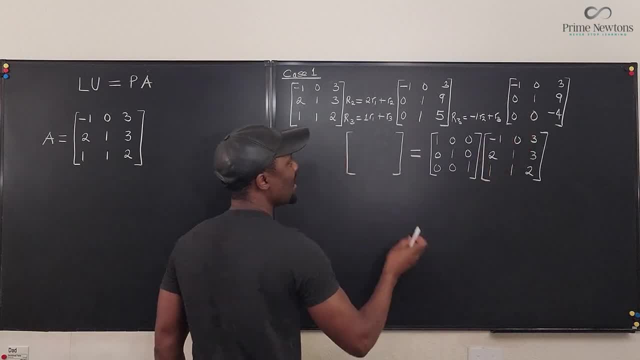 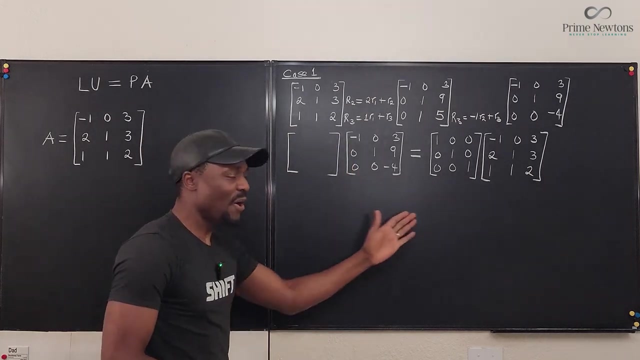 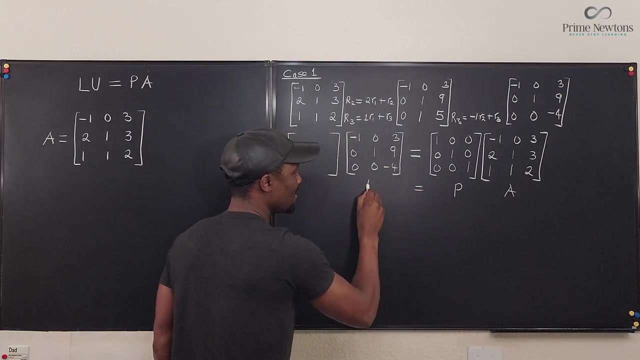 this is your U. your U is this thing that you got here, minus one zero three, zero one. nine, zero zero minus four. and tell me what is my L. you see how easy this is. so now I've got my A, I got my P, I got my U, and what do I have? 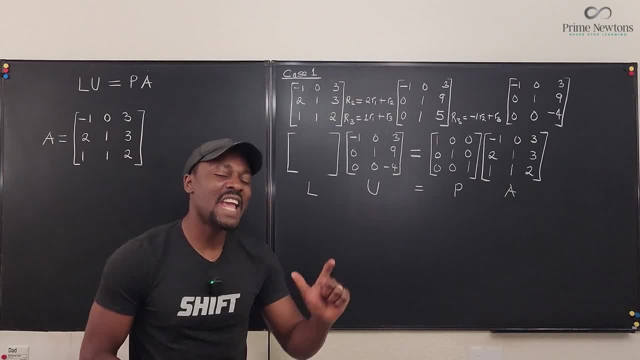 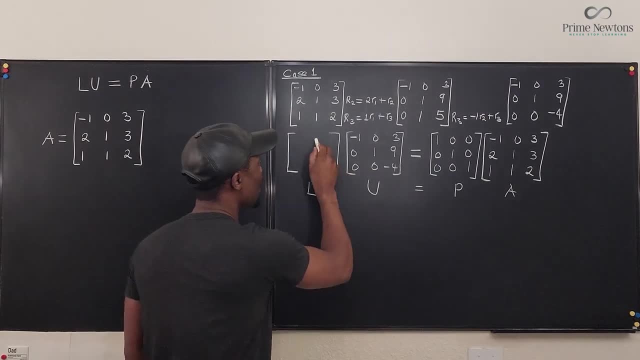 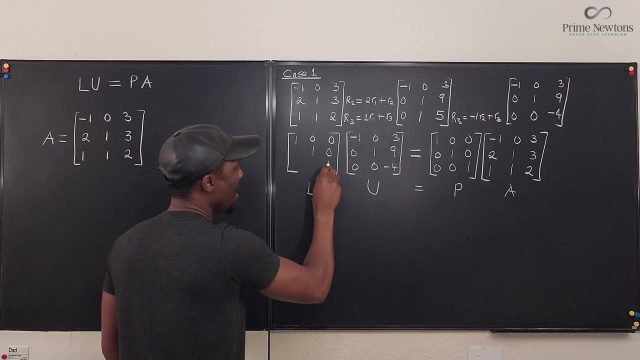 here is L. L is called a lower triangular Matrix. it means everything above it is a zero. so we're gonna have zero, zero, zero. we have one, we're gonna have one. we're gonna have one, we're gonna have one. that is how you start. there are only three numbers you need, because this is a three by three matrix. 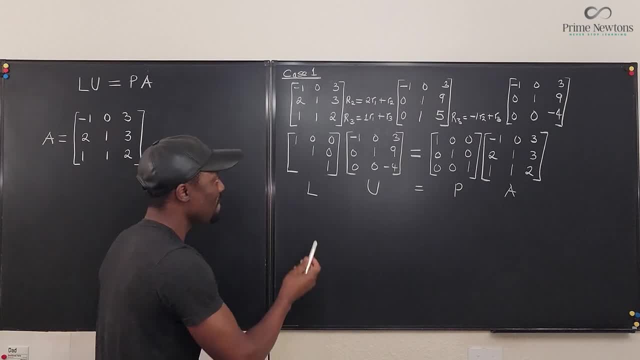 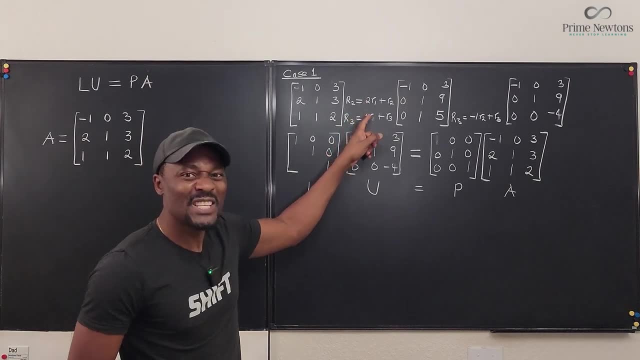 or at least you did three eliminations. okay, now you need to put numbers here. the numbers you put here are the numbers that undo the things you did here. so what did you do here? you needed positive two of r one, which was the pivot here. so because you needed positive two of it, you go put minus. 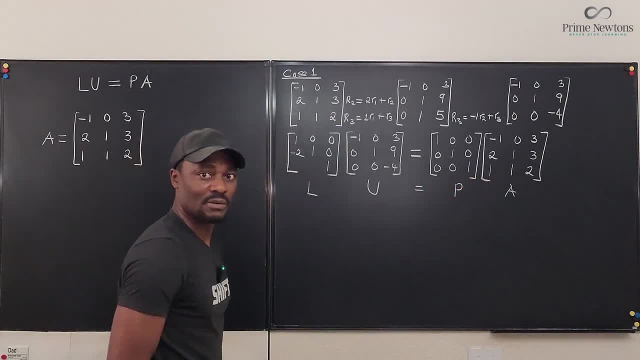 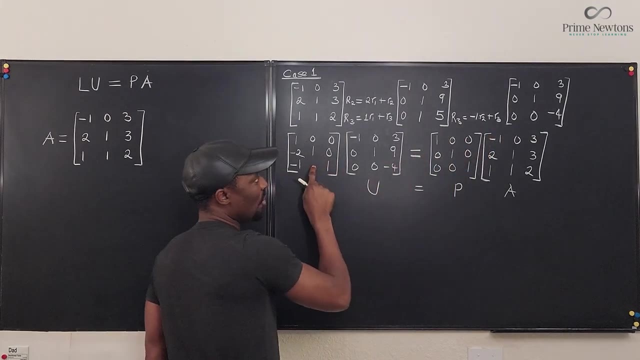 two of it so it can undo it and take you back to the original. so you go here because you needed positive one of r1 here in this row to make this a zero. you can see, to generate the zero, you go put minus one here and here. when you got to this point, what did you do in order to make this a zero? you? 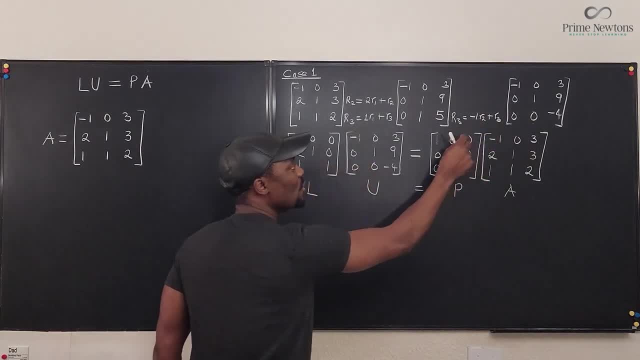 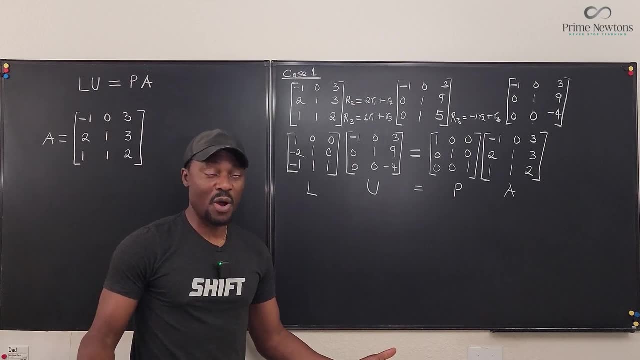 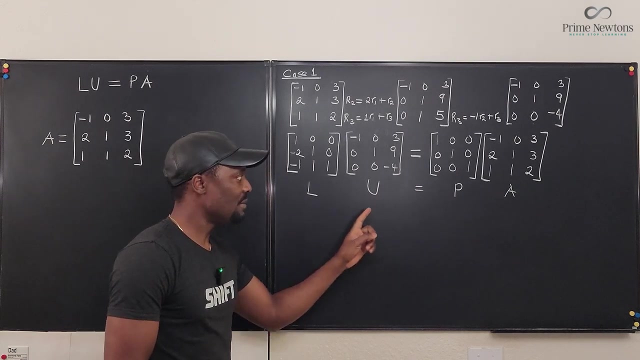 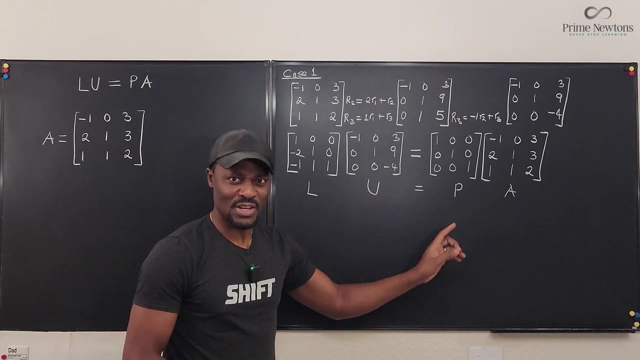 needed negative one of r2. so now you go back here and you go put a positive one, you have generated all the matrices required to fulfill this equation. this is the decomposition of this matrix. so it's like saying three times four is equal to one times twelve. because this actually is your one, let's 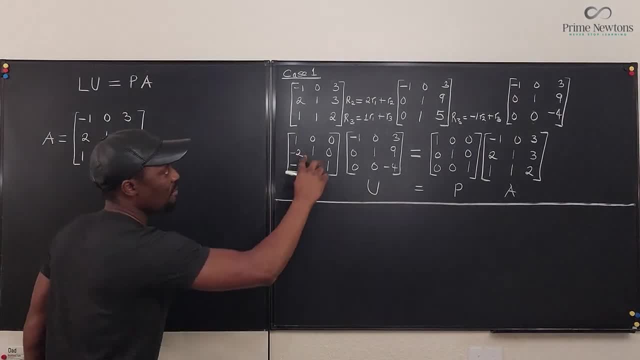 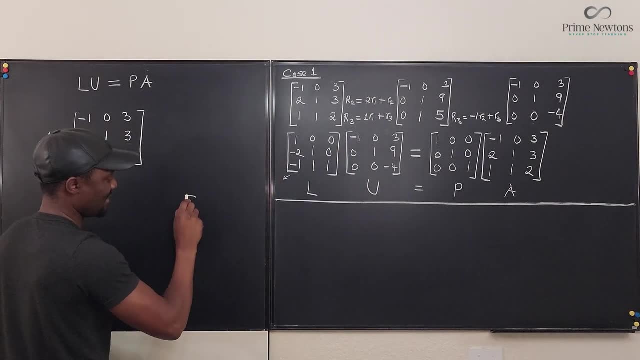 test that out here. let's do that here. so if i multiply this by this, what do i get? i'm gonna get minus one here. i'm just gonna do the solution to this here. okay, if you can test it quickly: one zero, zero times minus one zero zero. you get minus one. one zero, zero times zero one zero. you're gonna get um zero here you. 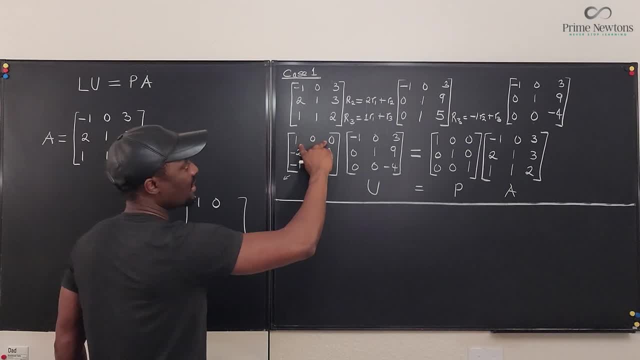 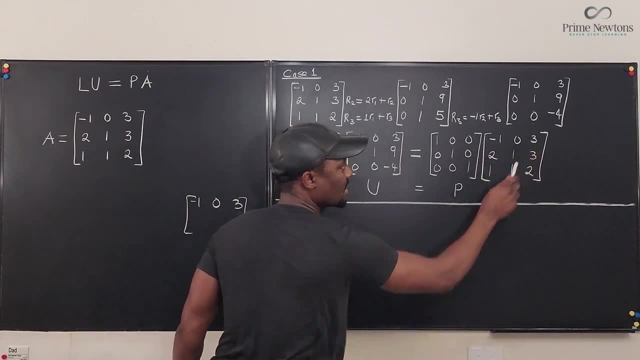 get zero zero, oh zero. you multiply this by this, you're gonna get three zero zero. that's three minus one zero three. does it conform? oh, it's the same thing we got there. let's go to the second one. if i multiply this by the first column minus two times, 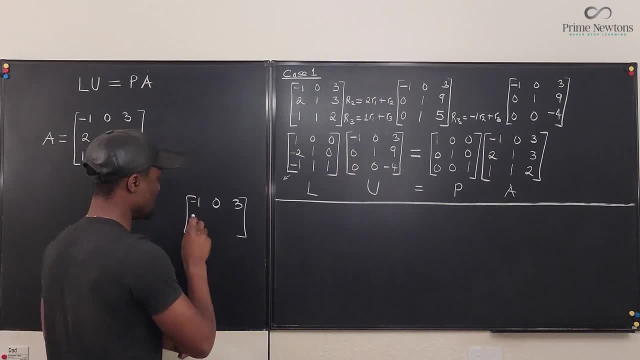 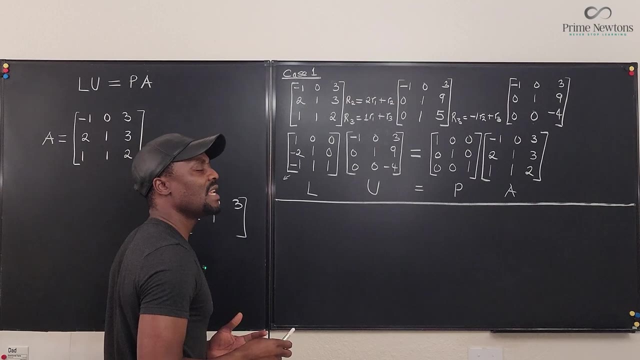 minus one gives me two. everything else is zero, so this is two. if i go here, i multiply, this is zero. this is one. this is zero, so it's just one. if i multiply this way, this is going to be minus six. this is nine. this is zero. minus six plus nine is three. this is three. okay. 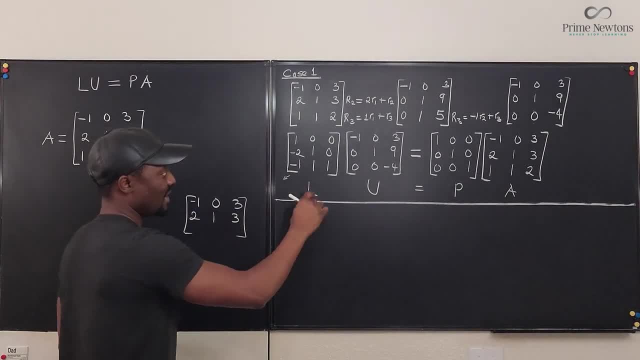 two one, three, two, one, three. correct, let's go down here minus one, one one. use it to multiply this: this is going to be one. everything else is zero, so this is one. if i multiply this way, this is going to be zero. this is one and this is zero, so it's just one. 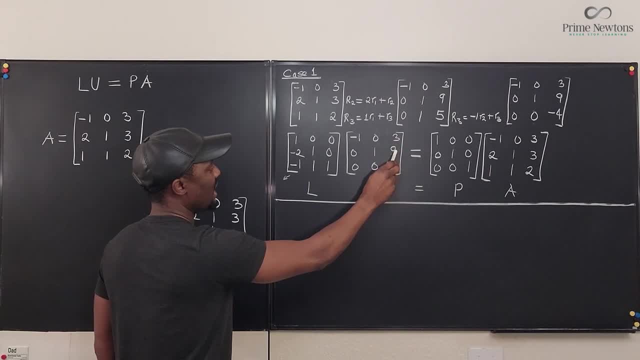 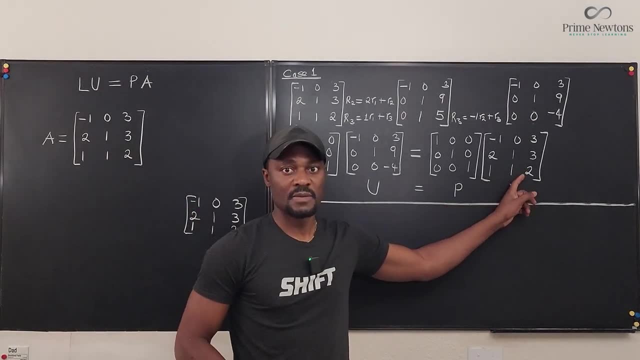 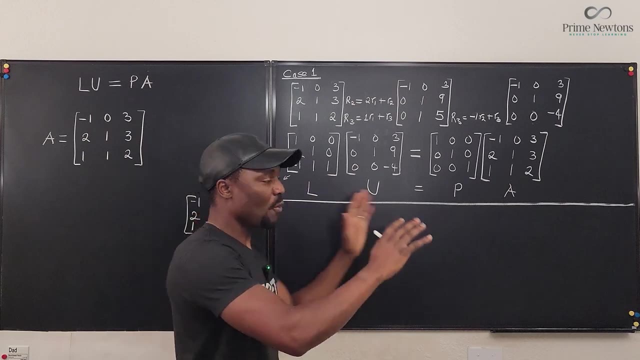 and if i multiply this this way, it's minus three plus nine minus four, so that's minus seven plus nine, which is two one one two. that's it. and notice that if you multiply, this is the identity matrix. you multiply this by this. this is what you're still going to get. so what we did is correct. 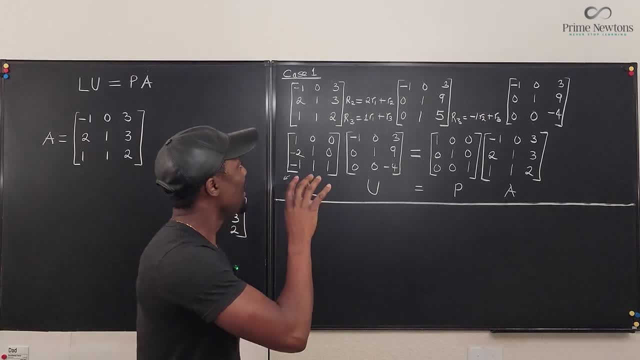 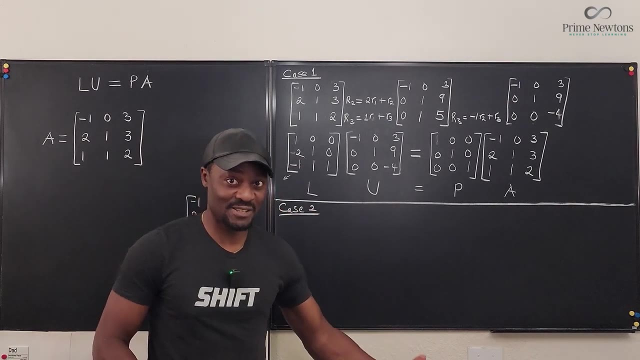 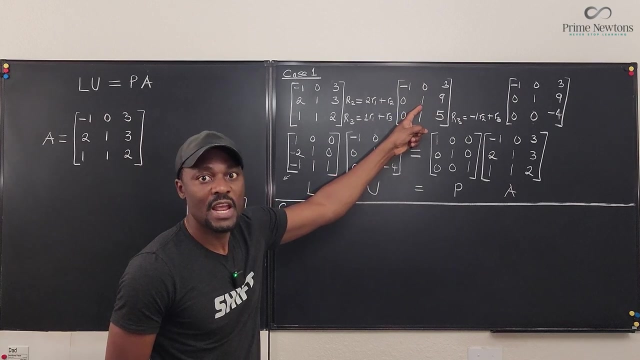 now let me show you what happens when you choose to switch rows. okay, if we choose to switch rows, case two now. sometimes you choose to switch rows. sometimes it is necessary to switch rows because you don't have an anchor. look at here, i had an anchor. here i had a one. assuming there was a zero here, it would. 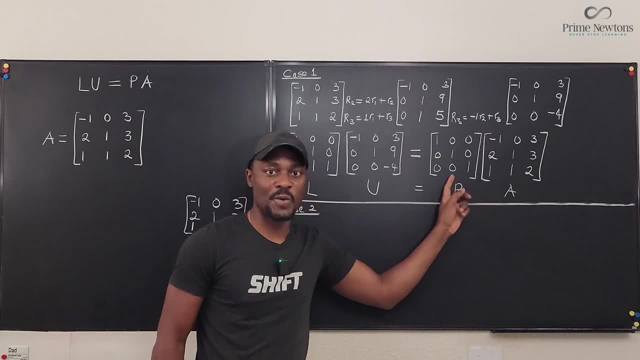 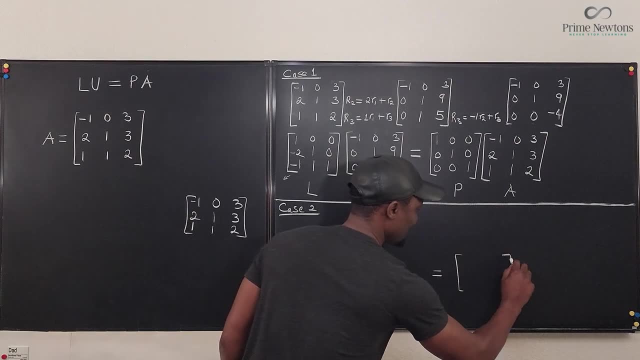 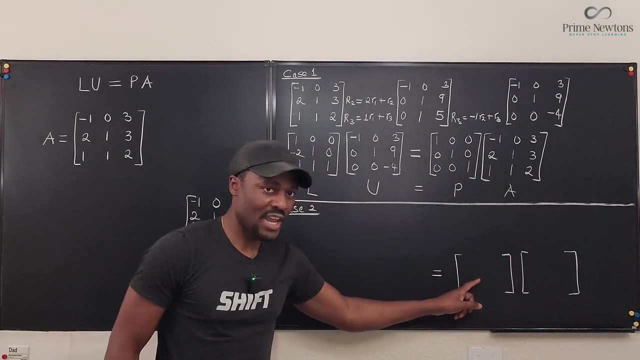 be mandatory for me to switch these two rows, and then you go show it here, so let's go. i'm gonna say that, in the final analysis, we're gonna have our p and a. now this is going to change. if this changes, this will have to change. okay, because this can no longer be. 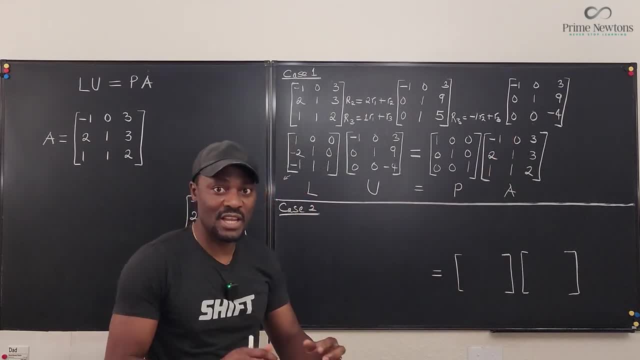 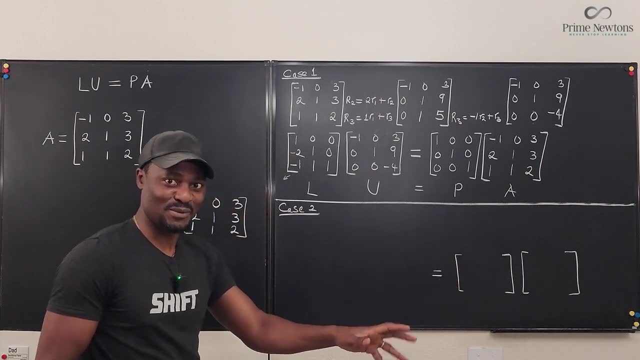 the original. once you change this, it's like saying you're changing 1 times 12 to 2 times 6.. you can't say 2 times 12 again. you have to change the 12 to a 6.. so let's go here. 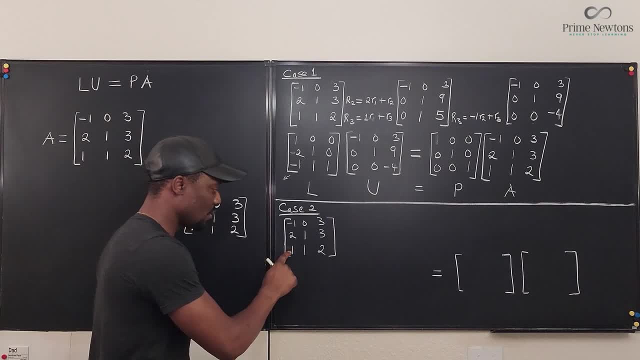 so i've got the original matrix here and i'm going to. i want this one up here. i don't want this minus one. we don't like minuses at the beginning. okay, let's start well. so what i'm going to do is i'm going to work on this and say that this row one is going to be switched. 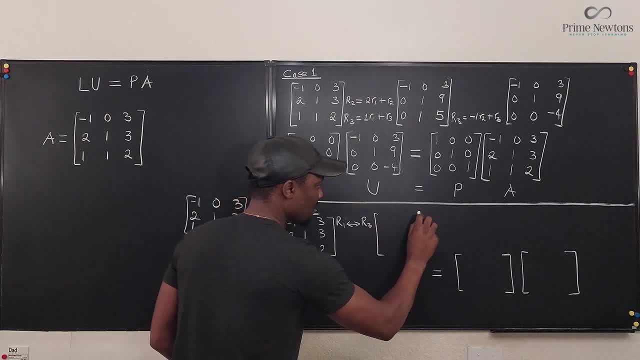 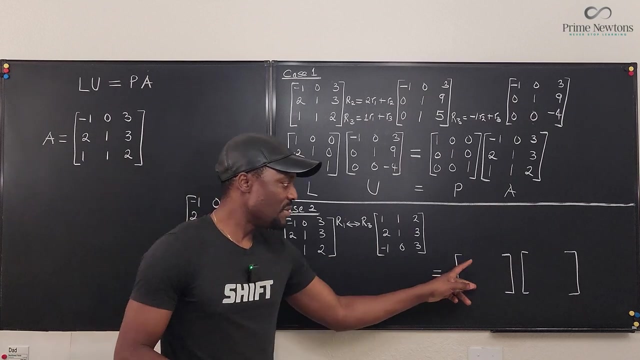 with row three. so now i have a different matrix and my matrix now looks like this: one one, two, two, one, three and i have negative one, zero, three. because i have done this switch, i have to immediately go here and switch the first and the third rows. okay, so i'm gonna go do that. this is gonna be zero, zero one. 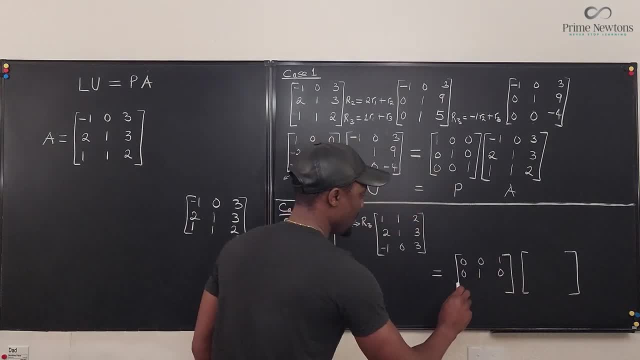 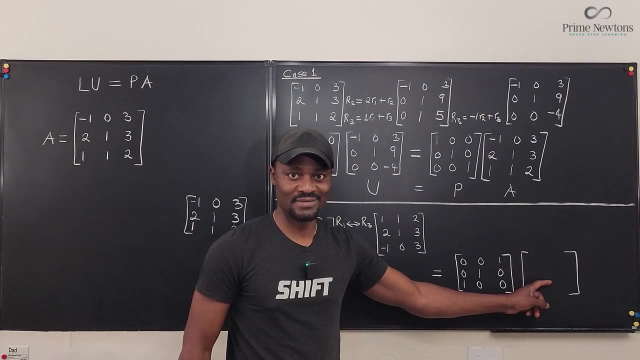 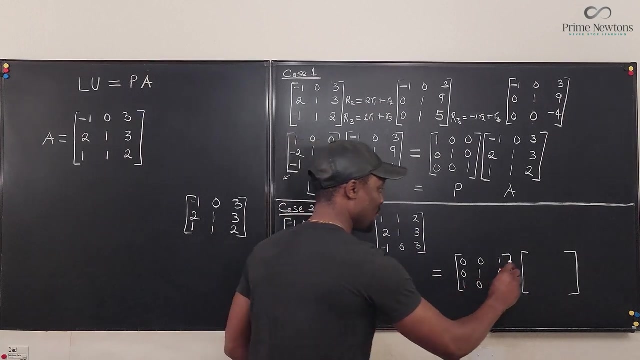 now, and the middle stays the same and the bottom becomes one zero, zero. okay, now what will be here? this new matrix you obtained after performing a row switch what becomes your a remember? you could use this to switch it back to this. that's what we do. so what I'm gonna do is I'm gonna write this as my one one. 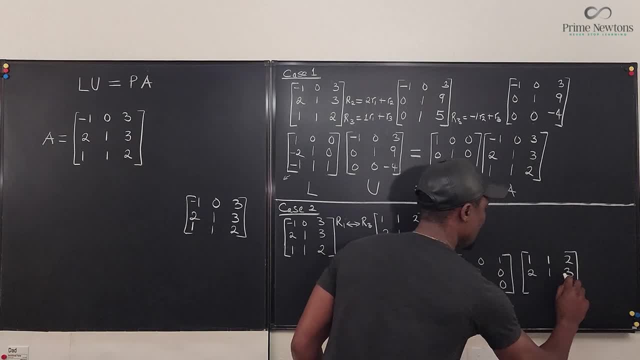 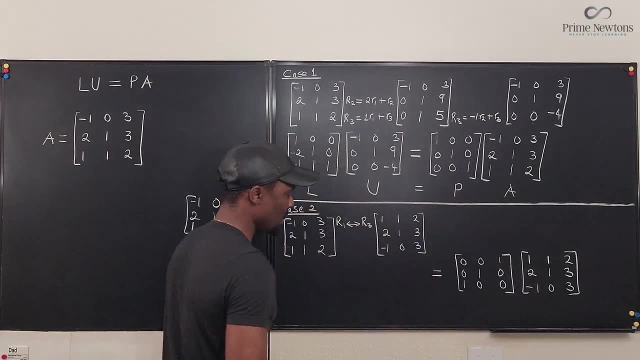 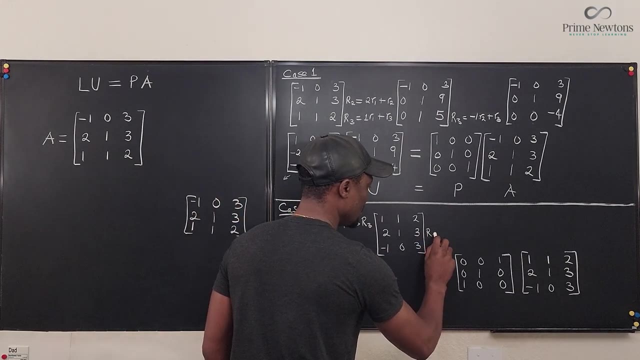 two, two, one, three, and this is minus one zero three. we're gonna go here and say: what do we do? I want to make zeros here. so if I want to make zeros, what do I do? I know that this row two is equal to minus two of this, minus two of row one. 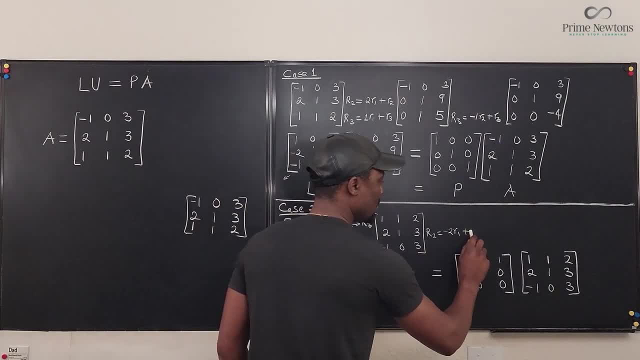 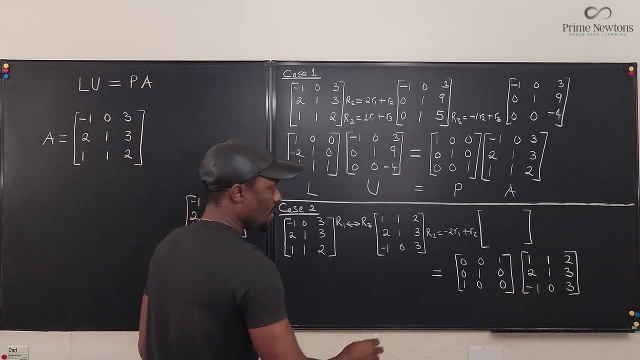 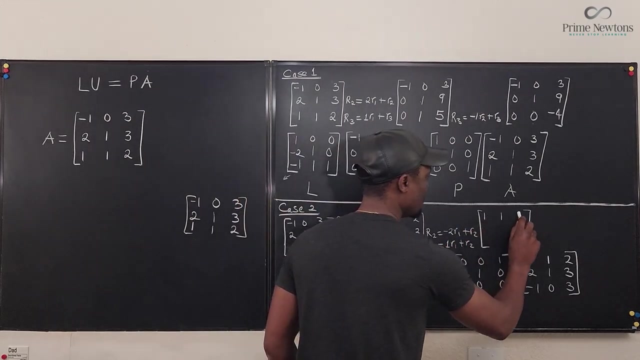 added to row two. okay so, and if I want this, it's gonna be: row three is equal to this, added to this. it's just one of row one added to row two. so let's write our answers: one one, two. what do we have here? we're gonna get a. 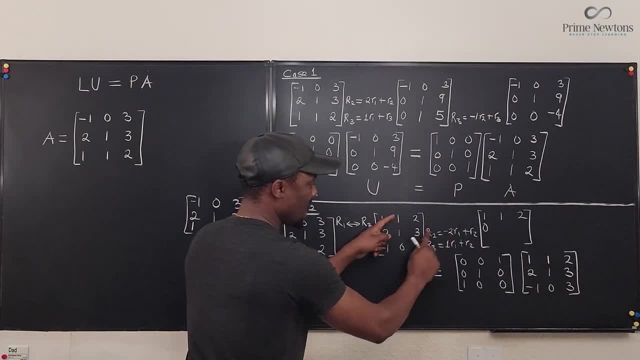 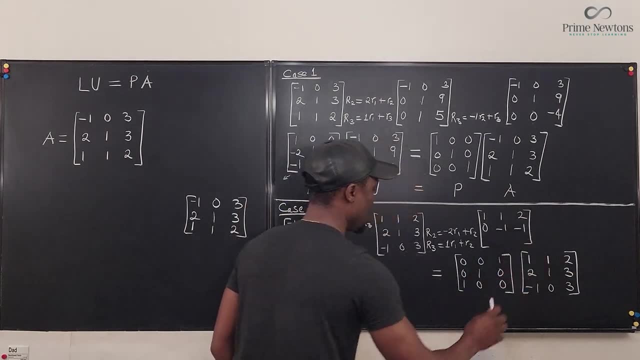 zero here. this is minus two of this added to this. so minus two plus one is minus one. minus this, minus four plus three is minus one. nice, and here we're going to have this plus this, so it's um. this plus. this gives us zero. this plus. 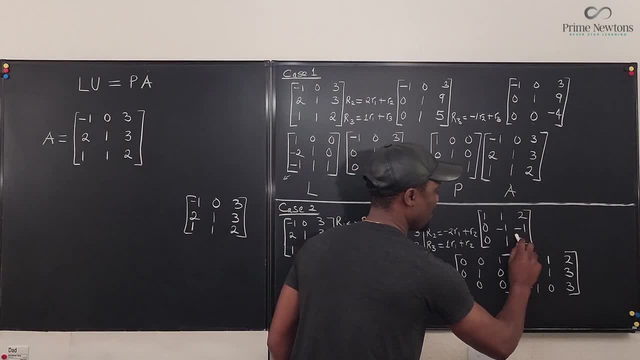 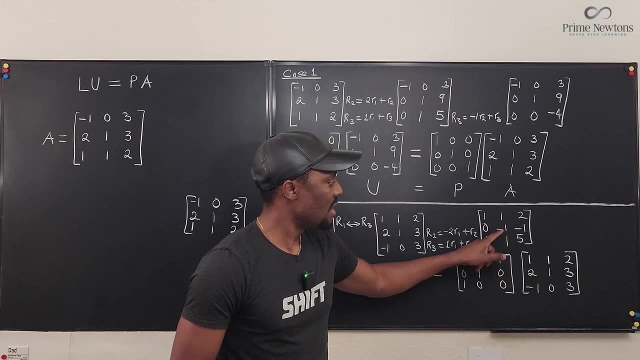 this gives us one, and this flows, this gives us five. Okay, one more move. we need a zero here. And how do we get a zero here? if this is our pivot, It's gonna be: just add these two together. So we're gonna say for row three: 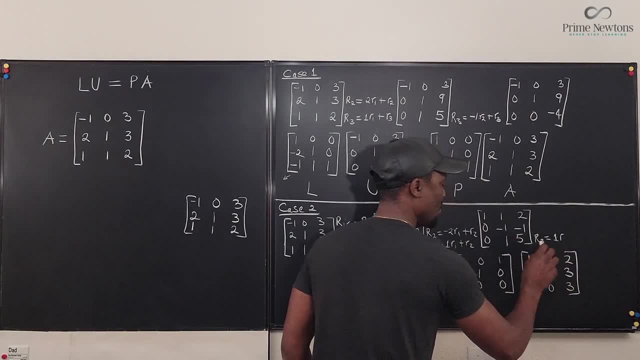 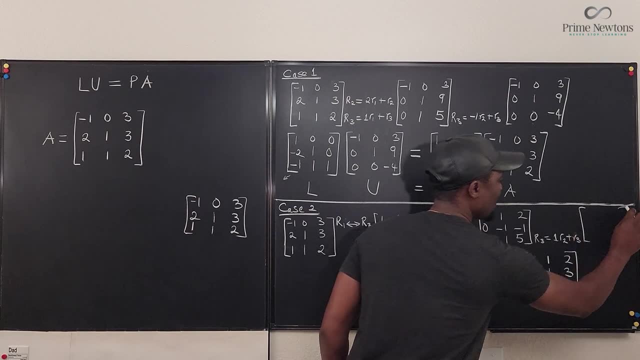 it's gonna be one of row one of row two, rather, add it to row three. Okay, I'm gonna squeeze it here. We have one one two, one, one, two. this doesn't change. We have zero minus one minus one. 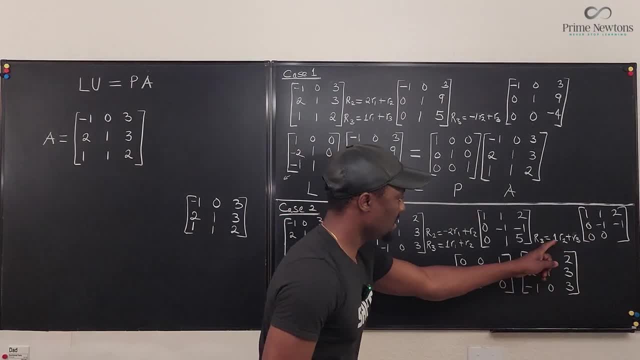 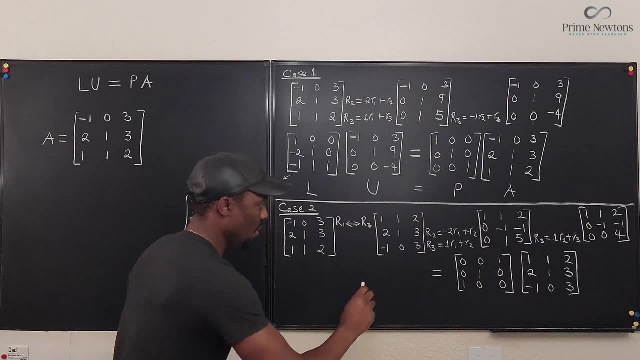 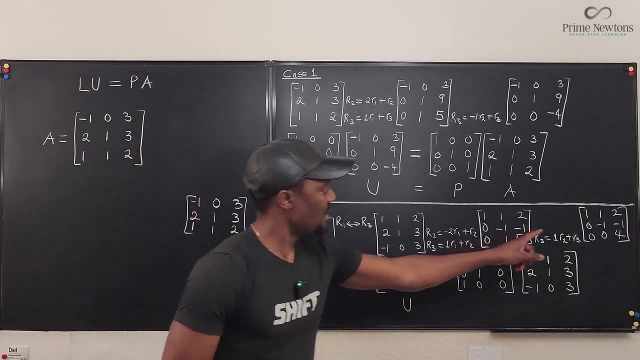 And finally we got zero. we got zero because, as the sum of these two, this is gonna be four. Okay, huh, we're done. Okay, so we can say: this is our U, Our U is gonna be this matrix: one, one, two, four, nice. 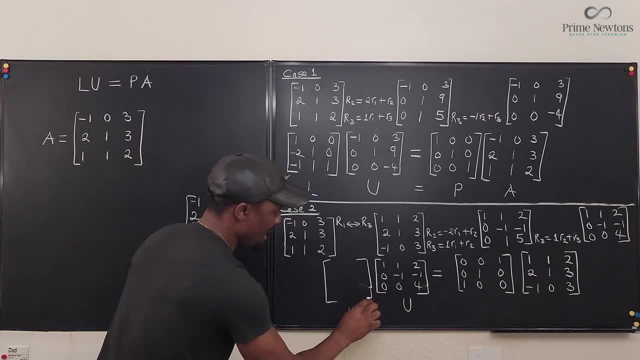 And this is our L. How do we get our L? Just go back to the eliminations you performed and undo them. Start by writing one zero zero, one zero, zero. sorry, What am I doing? One, and this is a one. 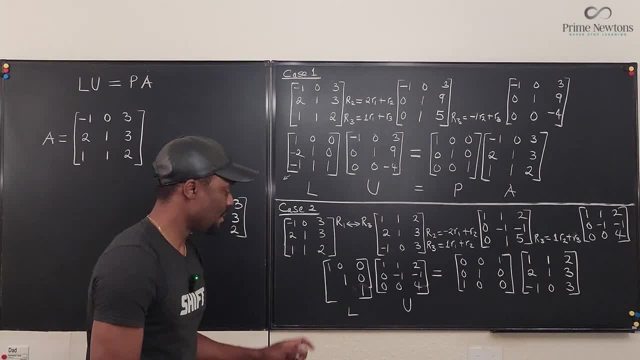 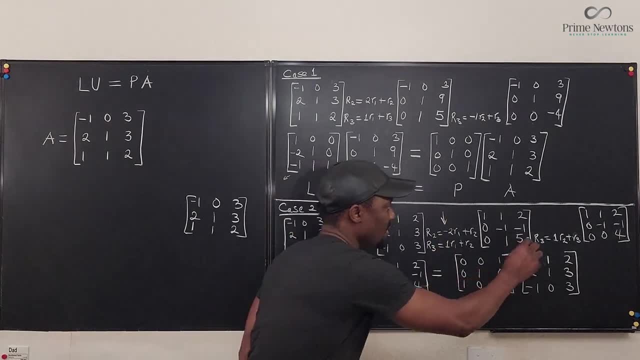 Okay, so we just need to fill two zeros here and one zero. I mean two numbers here and one here. So the numbers you fill in just focus on this part and this part. okay, What's the opposite of this? Where it's two, you're gonna add it back.